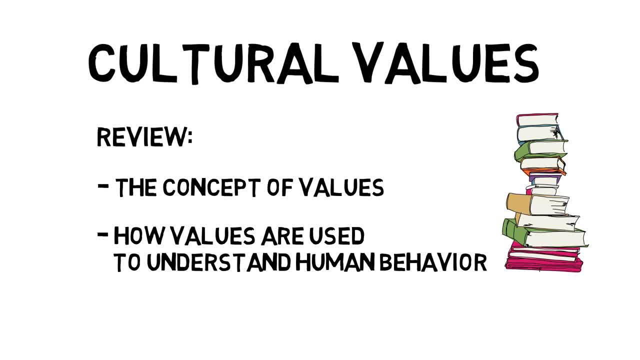 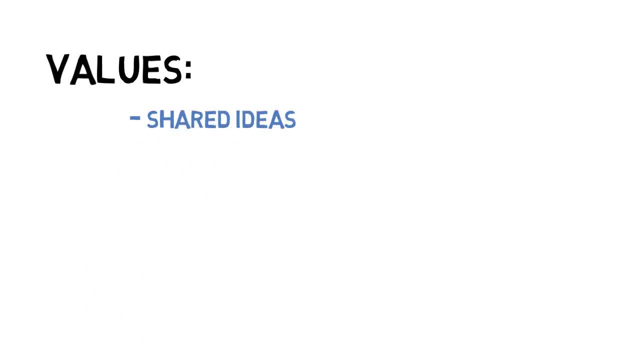 As the course progresses, many of the ideas discussed in this video will be covered in more detail. What are values? Values are shared ideas on what is good versus bad, ethical versus unethical, just versus unjust, reasonable versus unreasonable, and the like. 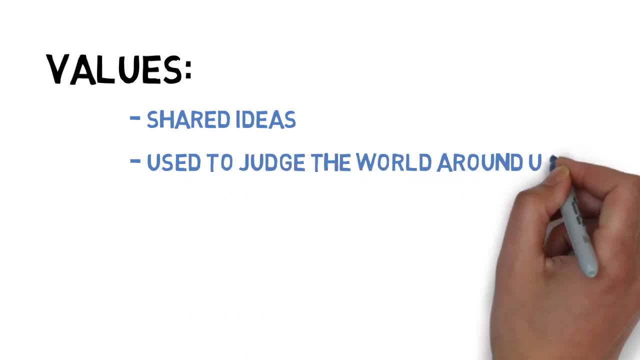 Values are what people use to judge the rightness or wrongness of what goes on in the world around them. In order to function and survive, societies create a collection of shared rules and norms based largely on their shared cultural values. Adults pass down what they know about proper communication behavior to their children. 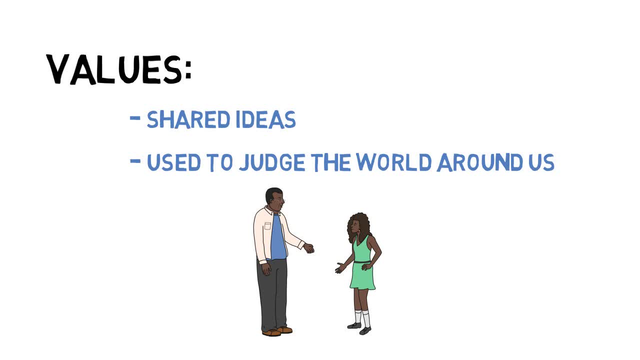 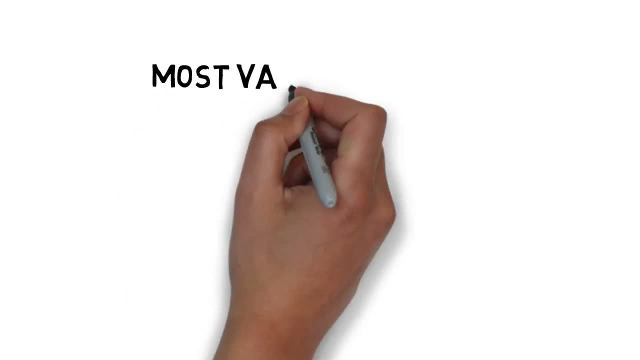 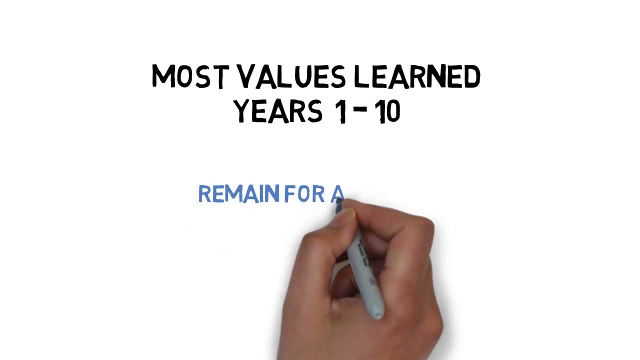 And as this passing down of knowledge continues through the generations, cultural values can persist within cultures for hundreds of years or longer. Most cultural values are learned before the age of 10, and once learned, it is difficult to unlearn them. The values we learn in childhood can influence the way we move through the world for the rest of our lives. 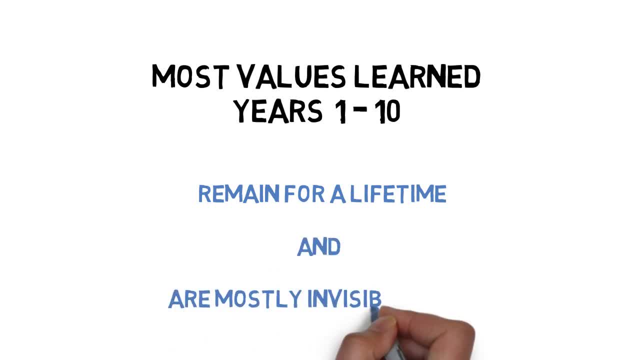 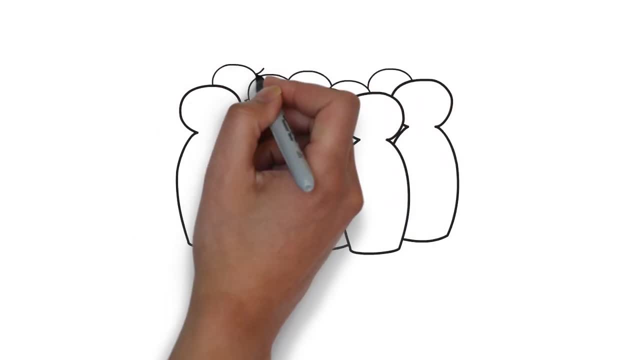 And since they are mostly invisible to us, we aren't even aware they influence our views. People tend to be drawn to others who behave similarly to them And who value and like the same types of things that they do. Humans have discussed this need for group-member similarity since ancient times. 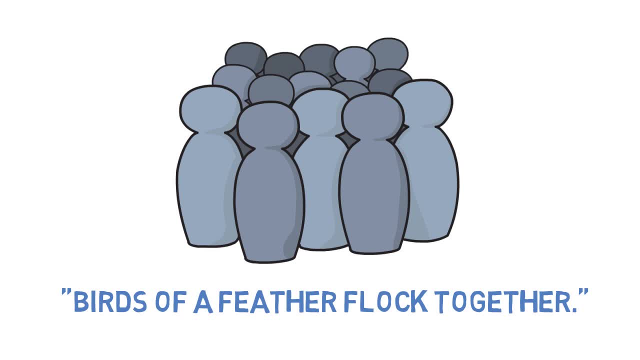 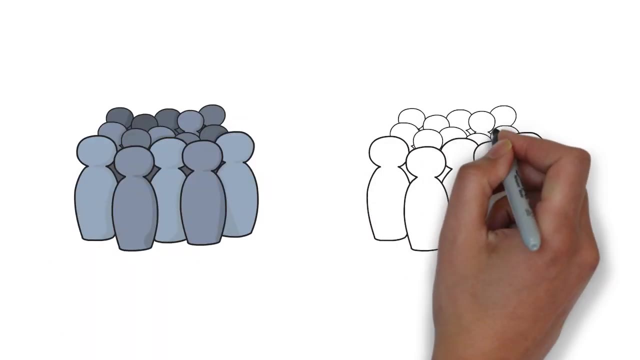 As the idea of birds of a feather flock together is mentioned in Plato's Republic. In fact, human connection is so important that much of an individual's time is dedicated to building relationships and maintaining group membership. Group membership can be separated into two general categories. 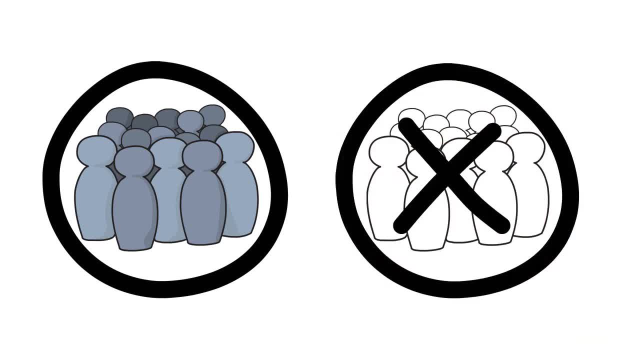 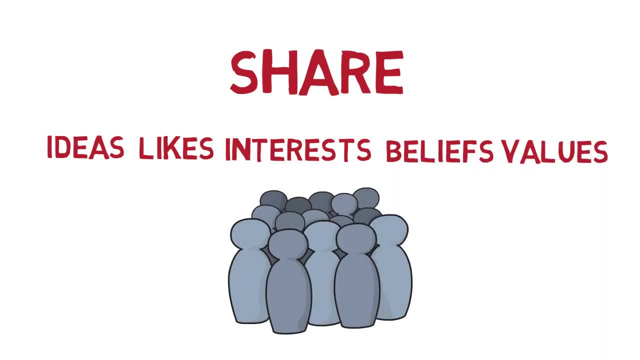 Those who are in your group and those who are out of your group. Those in your group are perceived as sharing similar ideas, likes, interests, beliefs and values. The similarities among in-group members draw them together. It is not uncommon for people in the same in-group to feel related, even if they are not from the same family. 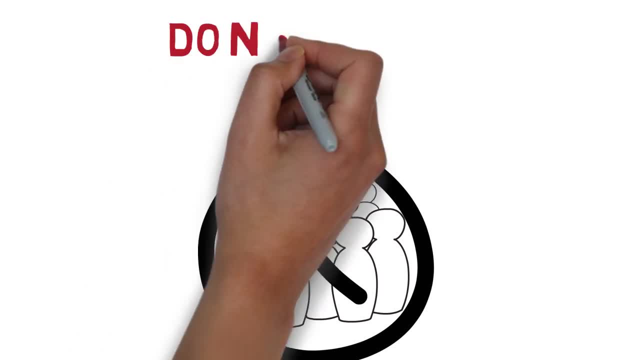 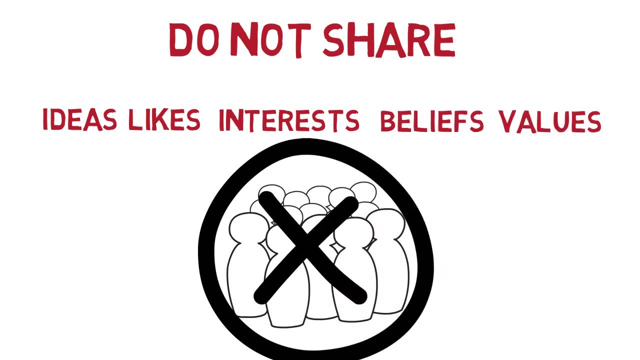 Those that are not considered part of your group are perceived as not sharing the same principal ideas, likes, interests, beliefs or values. Dissimilarity can be perceived as so significant, and the ideas in contention so fundamental, that people of out-groups are considered complete outsiders. 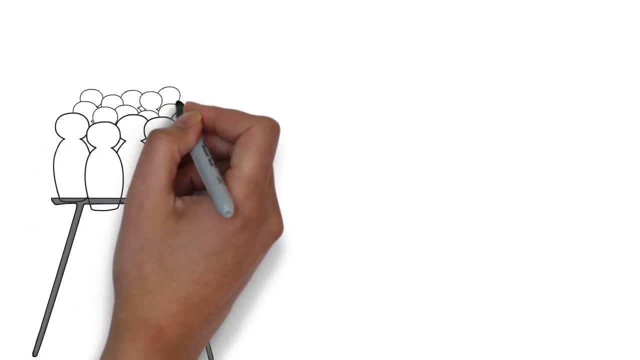 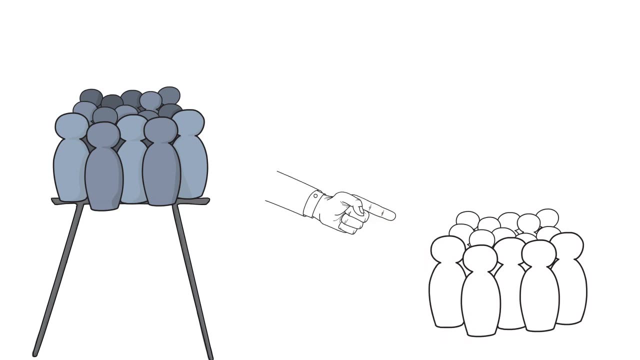 When it comes to making judgments on people's behaviors, humans tend not to use the same rules to judge in-group members as they do to judge out-group members. Only members of the in-group deserve full consideration, care, support, benefits and the like. 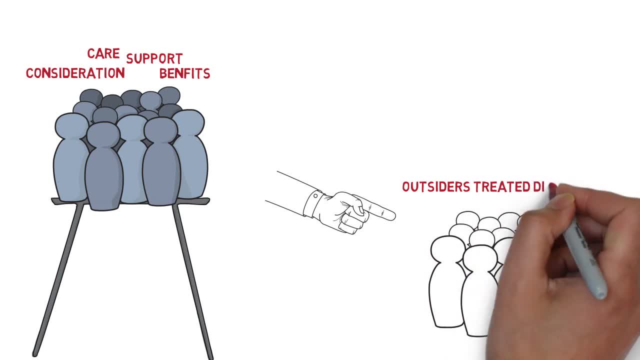 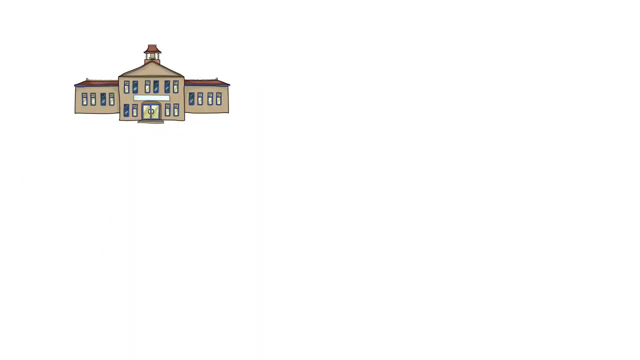 Those outside of the group are not entitled to these things and are treated differently. Understanding how obligations and beliefs differ for in-group and out-group members can help explain why contradictions seem to exist in belief structures. For instance, a government may claim that all people in their country deserve free health care. 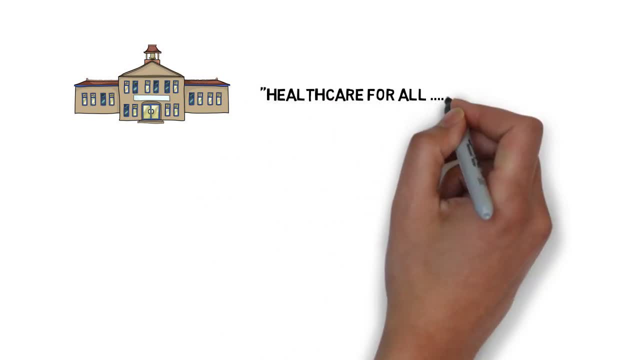 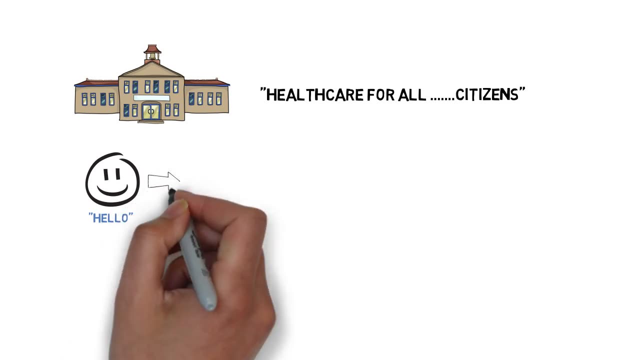 as it should be a fundamental right, but then only make it available to its citizens. Immigrants without citizenship should not receive the same benefit. A person may believe it's important to be polite when interacting with others, but is only polite to people who speak her or his language. 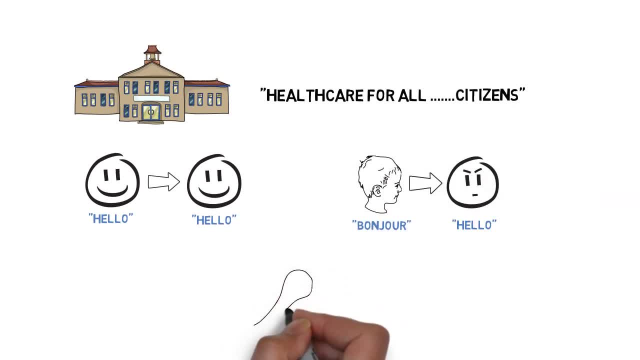 and is rude or cold to people who speak a foreign language Or a group may believe that people who are soulmates and truly love each other should live together, but only if the soulmates are comprised of one woman and one man. As humans, we belong to many groups. 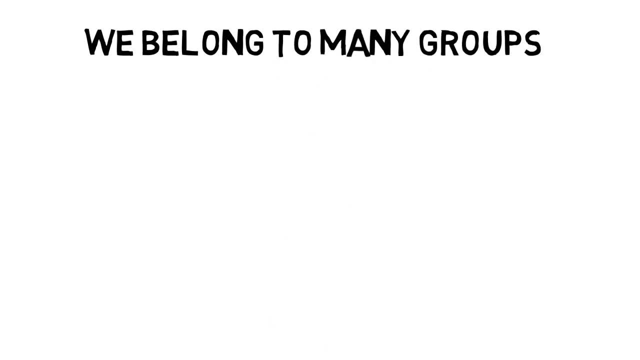 and some group ties are stronger than others. We can identify with national groups, ethnic groups, intellectual groups, religious groups, regional groups and even neighborhood and family groups, And when making decisions, each of our in-groups' values are considered, and only those for which we feel most connected to. 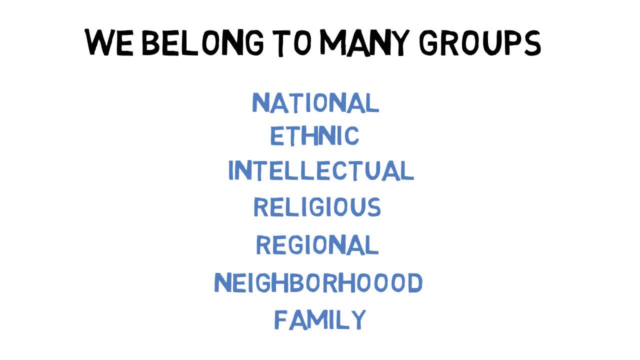 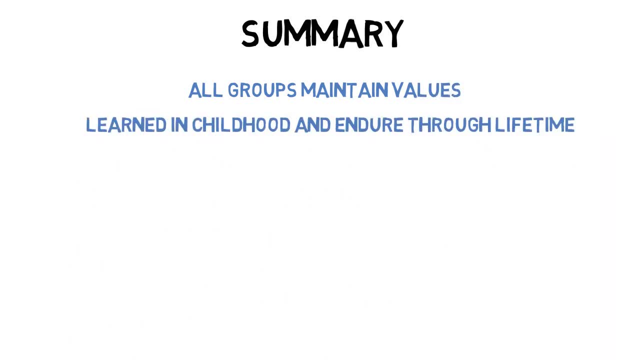 are given all the benefits, rights and considerations available. In summary, all human groups maintain values. The values are learned early in childhood and endure throughout a lifetime, influencing how people understand and judge the world and others around them. For the most part, the values we hold are hidden to us. 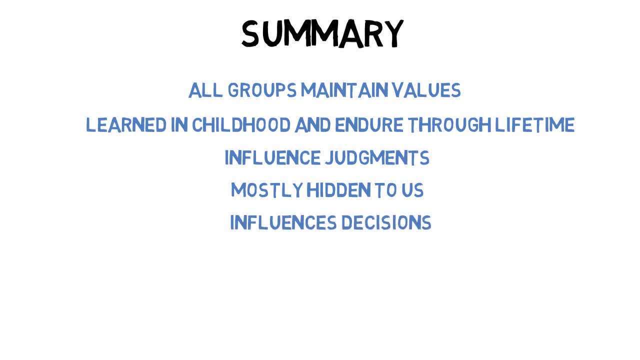 and work in the background of our thinking, influencing our responses to things around us. We align ourselves with people who seem to hold the same values as we do, forming in-groups, and see ourselves as different than those who do not share the same values. 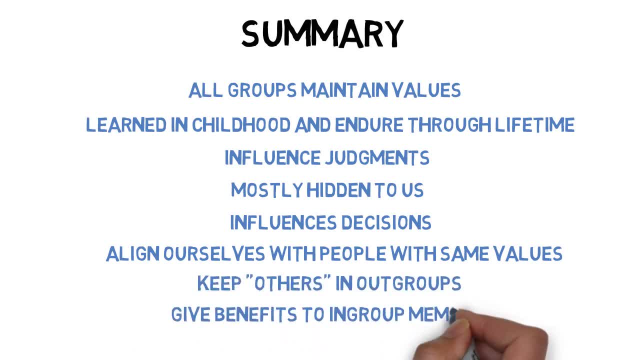 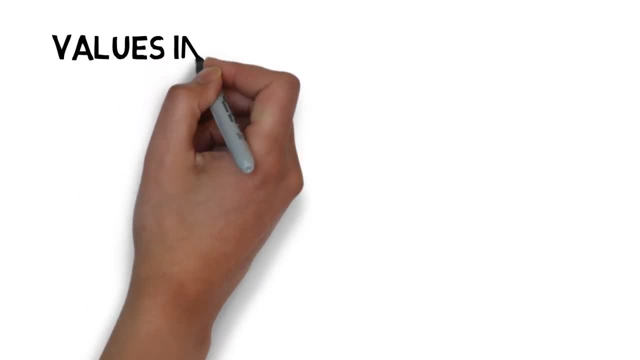 keeping them in out-groups. People do not feel obligated to give people in out-groups the same benefits, considerations or fair judgments as those in their in-groups. Knowing the role of values in the formation and maintenance of human societies and how value structures influence human behavior,